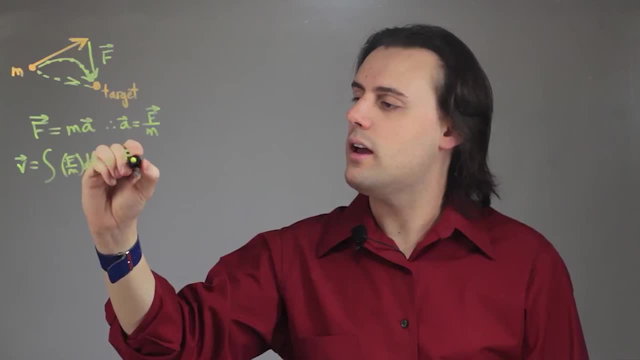 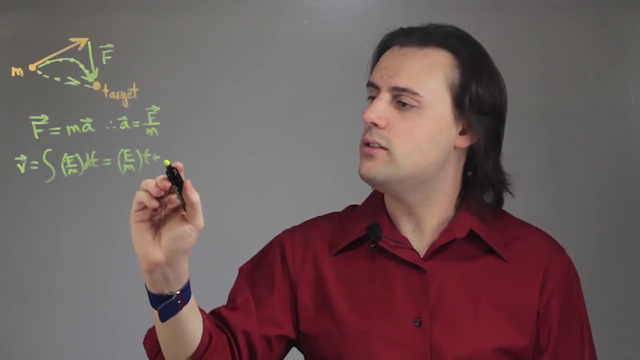 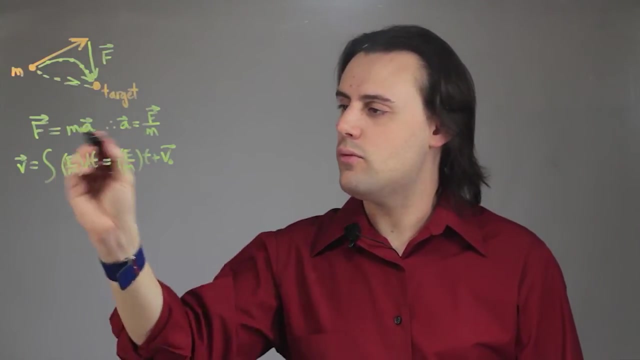 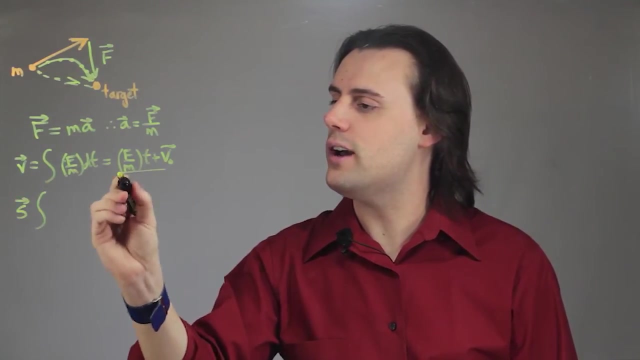 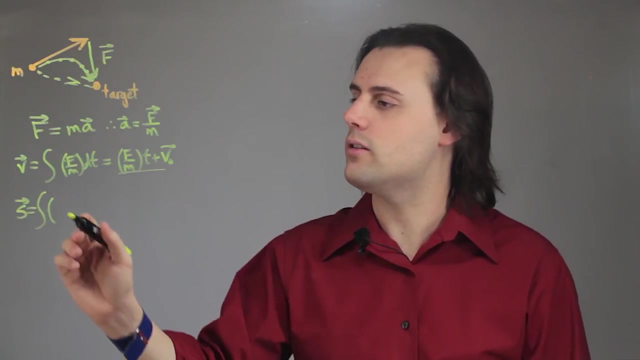 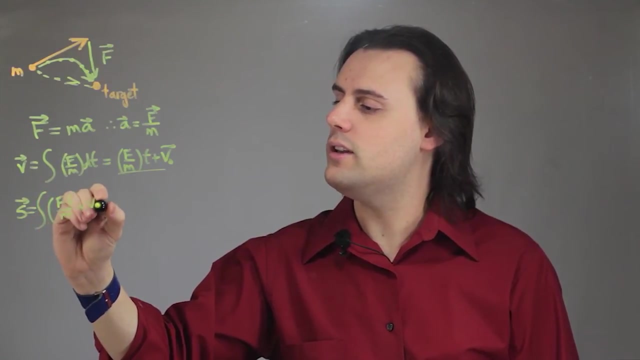 respect to time, and we get f over m times t, plus the integration constant which is interpreted as the initial velocity of the object. and then we do this one more time, we integrate the velocity expression we just found with respect to time to calculate the position vector, the trajectory. So we're going to have f, t over m plus v naught, and 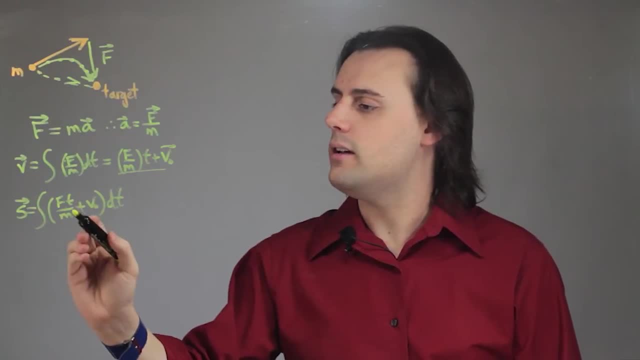 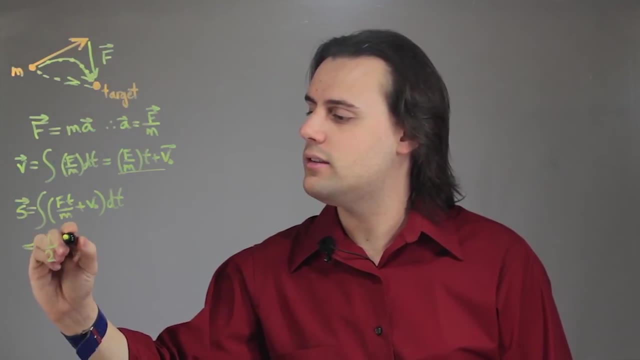 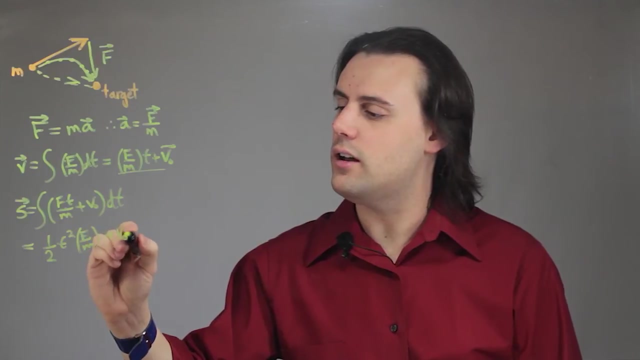 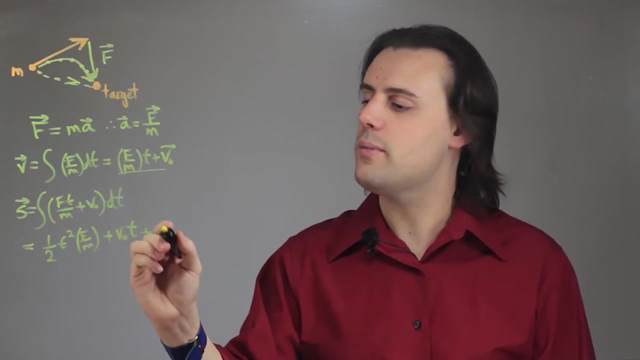 we integrate that with respect to time and because there is a linear t term here, we get one half t squared times f over m plus v, naught times t plus an integration constant which, again, like with respect to velocity, is interpreted as the initial condition here. 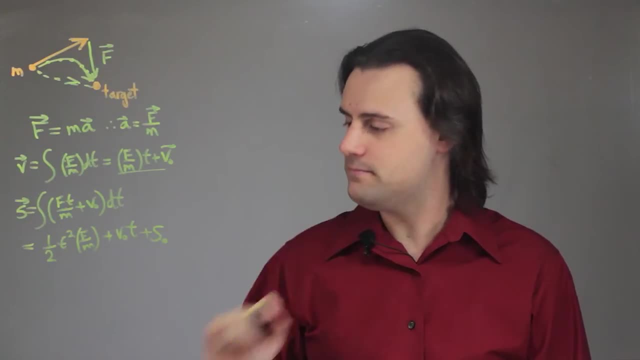 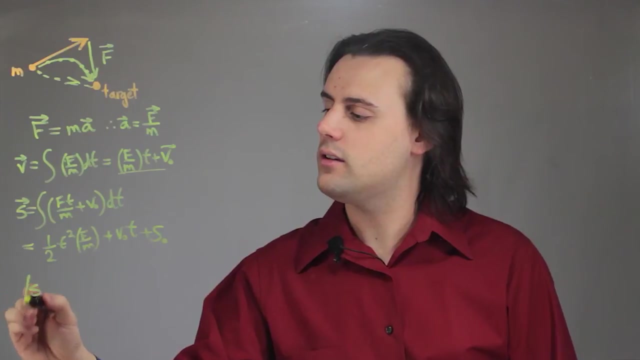 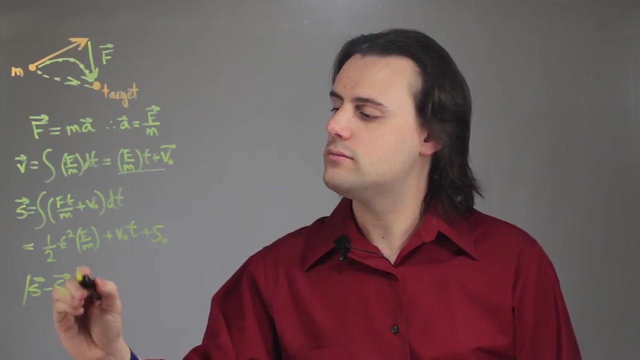 the initial position. So we end up with an expression for the distance t squared times f over m plus v naught times t plus an integration constant which, again, which is s minus s naught, is equal to. here I just brought the initial position over to. 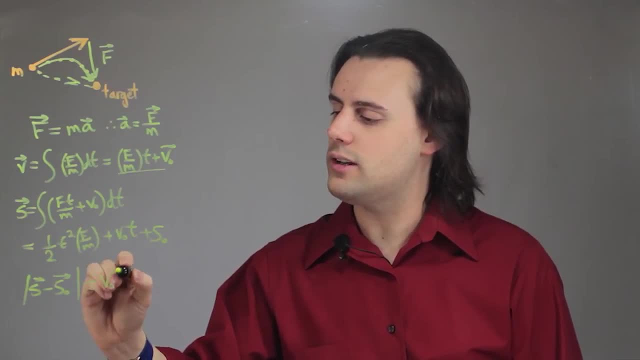 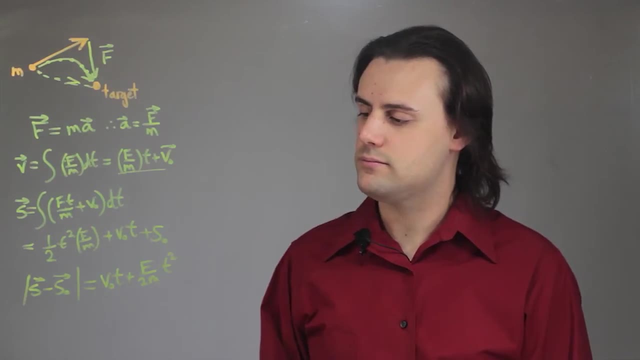 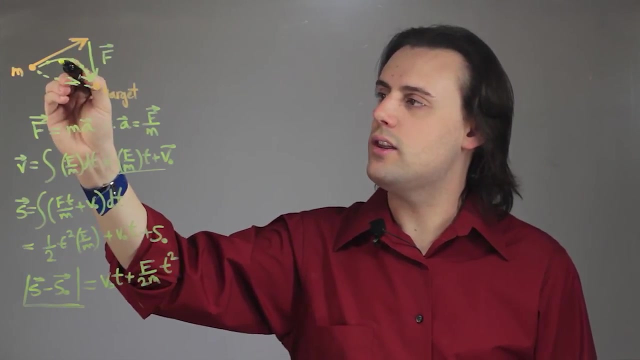 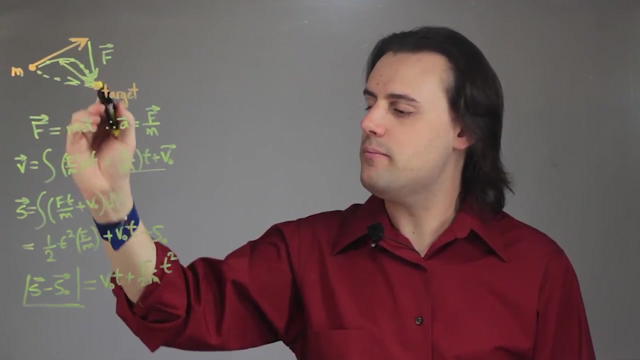 the left-hand side is equal to the initial velocity times time plus f, over 2m t squared. So you can view this as the separation at any point in time between the object, the mass and the target destination. So you can update this equation in time, provided you know. 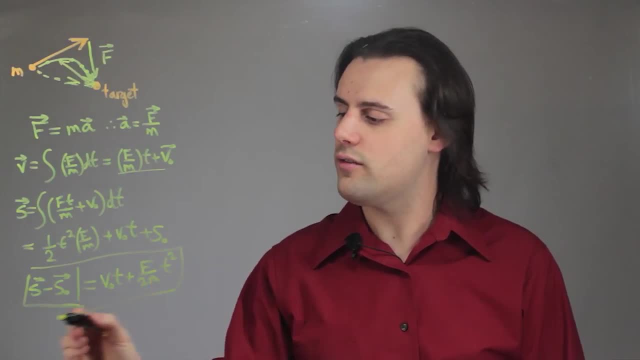 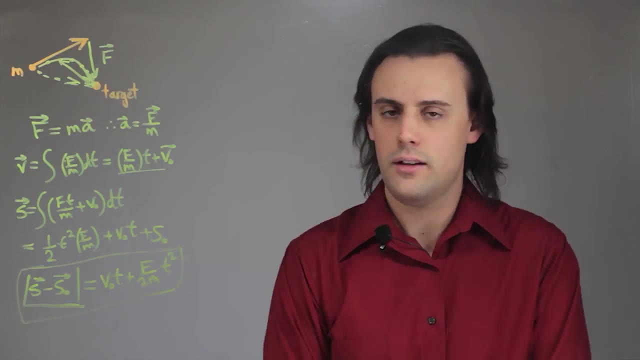 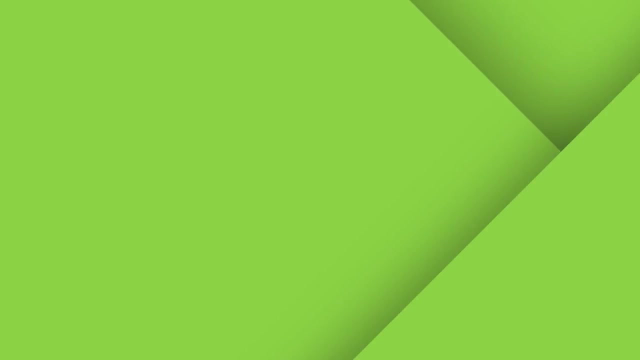 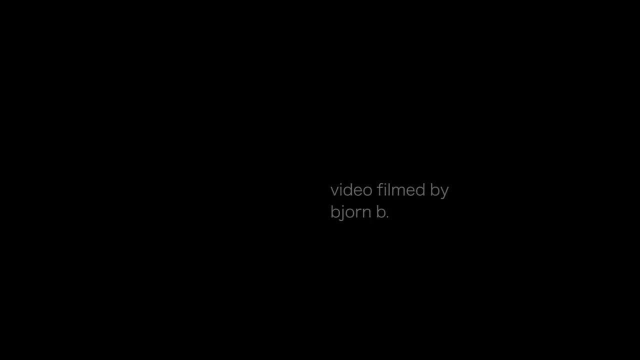 the steering force. this is an expression from kinematics for the distance, this separation distance that we're interested in. My name is Walter Unglob and this is how to calculate separation for steering force. Thank you very much for watching and I'll see you in the next video.